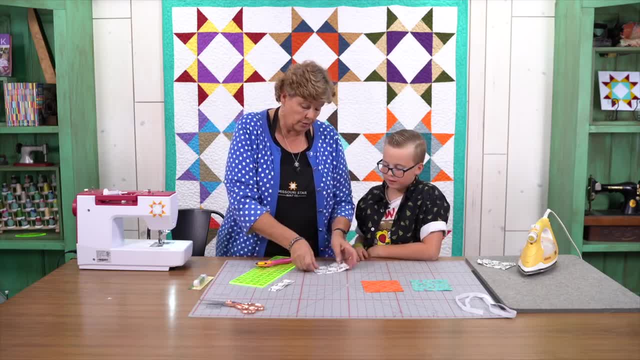 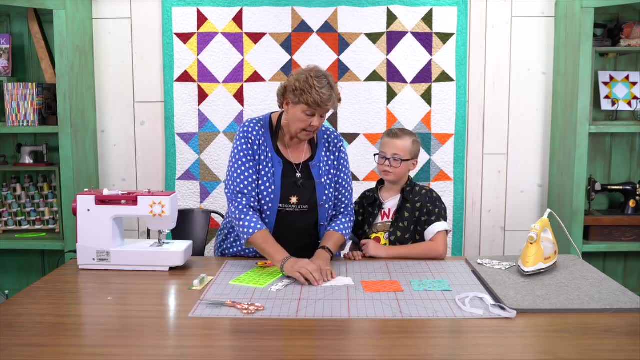 Yep, And what I want you to do now is I want you to take these two pieces and we're going to put them right sides together like this- Yeah, So facing each other, And I want you to sew a quarter of an inch all the way around. 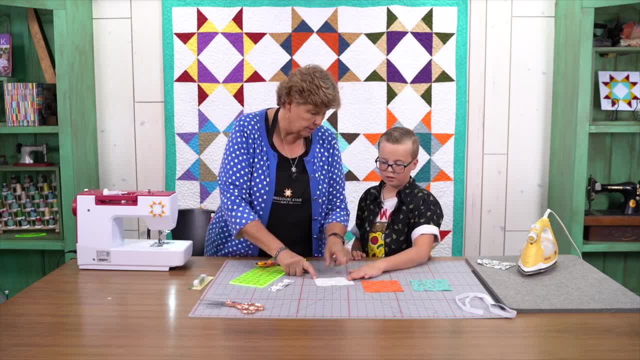 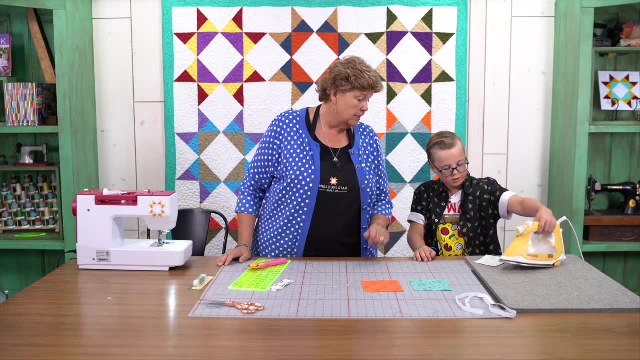 the outside. Alright, Let me- um, let's iron this little pleat out of here. Can you just go ahead and touch the iron and it will get hot And then you can iron that. so, because it's important that it's nice and flat, Oh, took it right out, Look at that. 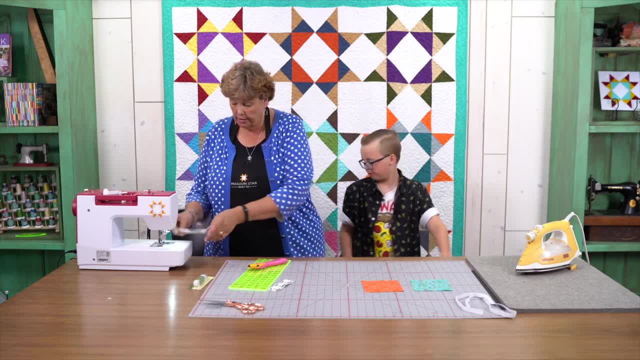 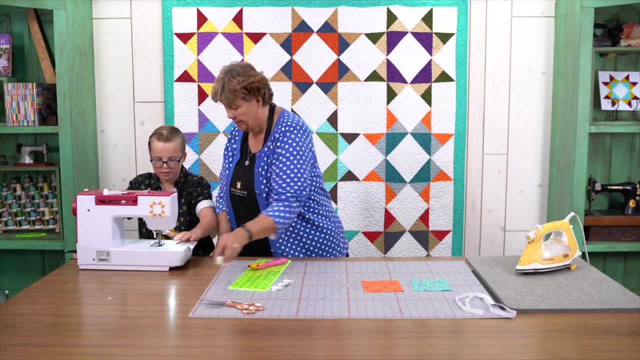 Oof Alright. So now we're going to go to the sewing machine. right here We're setting this up And Gideon- he has actually sewn some things before, so he's pretty confident here at his abilities And he's just going to sew around. 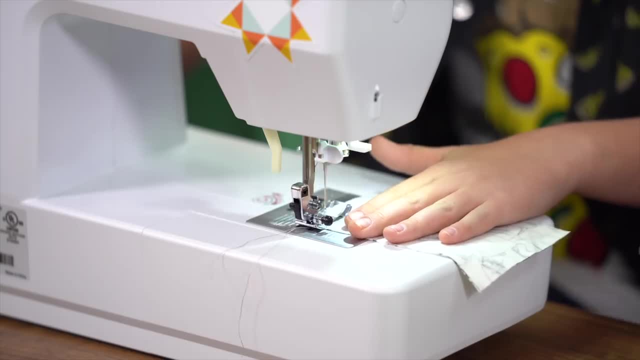 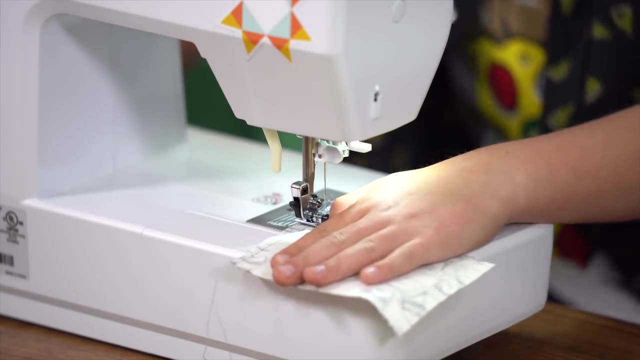 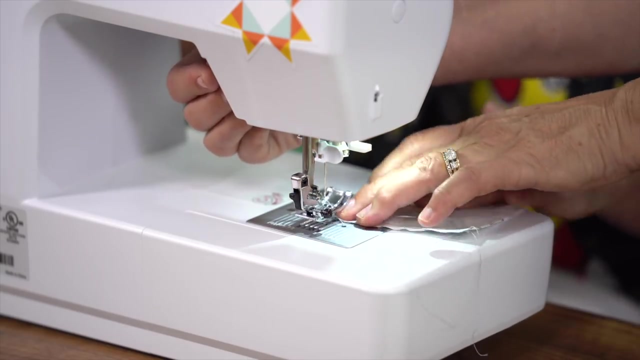 Yep, Go nice and slow. so your seams stay even And you can sew right off the end, or you can. you can leave your needle down and lift this up and pivot. Now, Gideon, where are you watching so that your needle can? um, I mean, where are you? are you lining it? 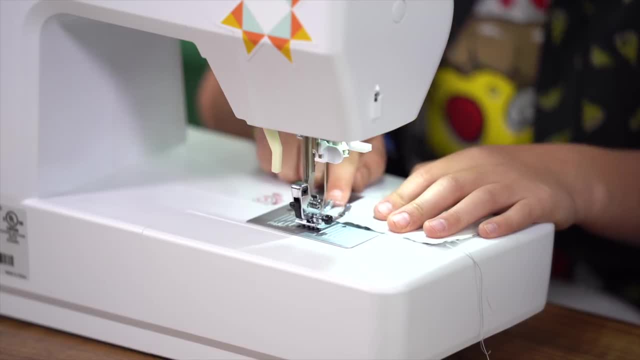 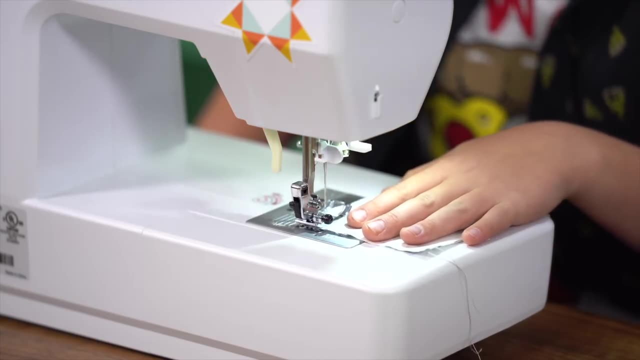 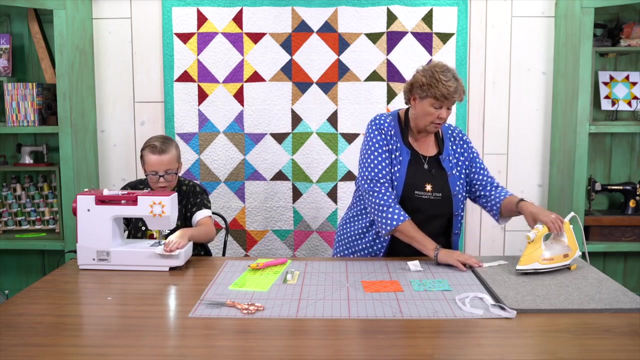 up along the inside edge of this. Yep, No, Yeah, OK, I think. Perfect, So watch, so this fabric stays right along that silver toe. Alright, While Gideon's doing that, I'm going to take one of these one and a half inch pieces that we have off. 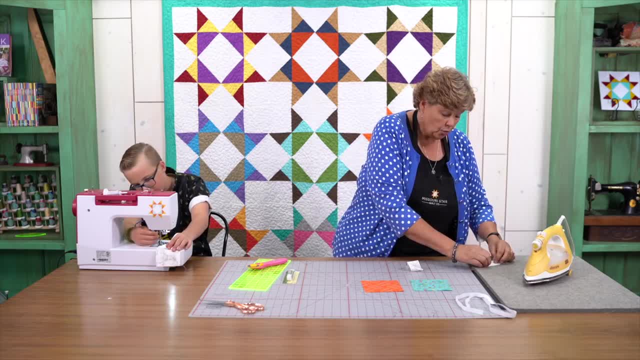 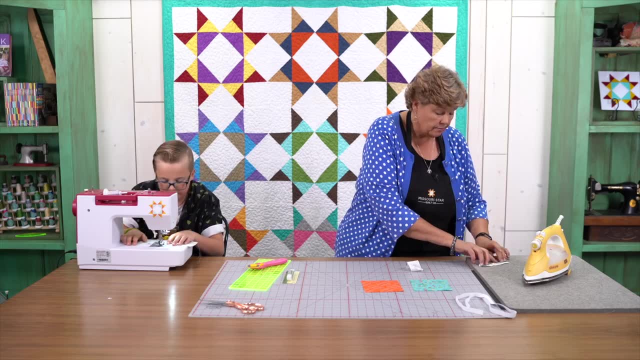 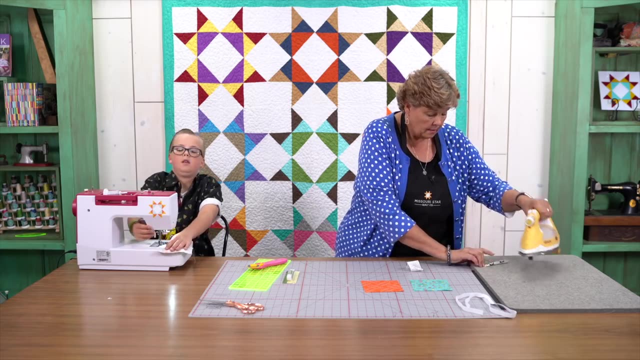 and I'm going to iron it to the inside. So I'm going to fold it in half, like this, And then I'm going to fold the two pieces into the center, like this, And one more. So I'm going to press the edge. pressed to the side, away from the edge, a little bit Enough. 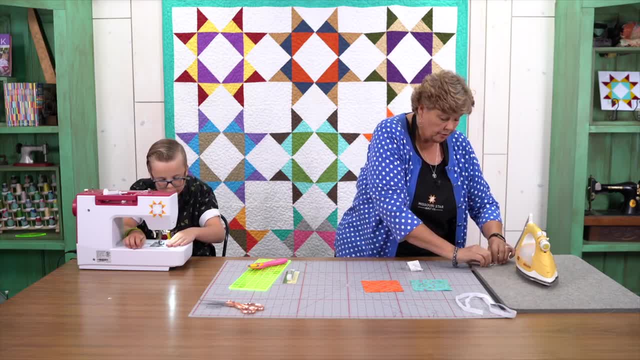 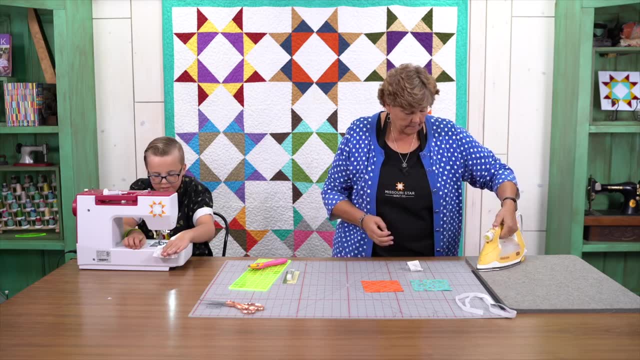 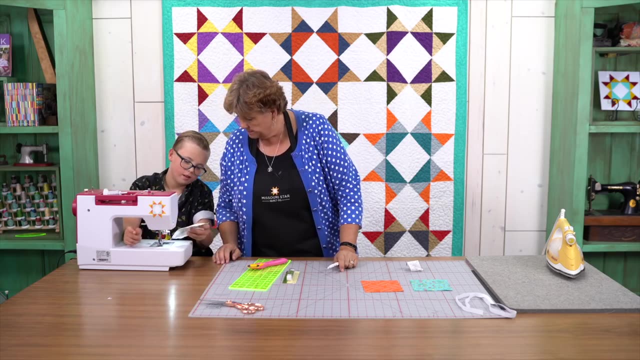 patience. Just press a little more, OK, And then I'm going to fold it in half again. How are you doing? I think I'm done, You're done, Awesome, Alright. now what I want you to do is see, I have this little. 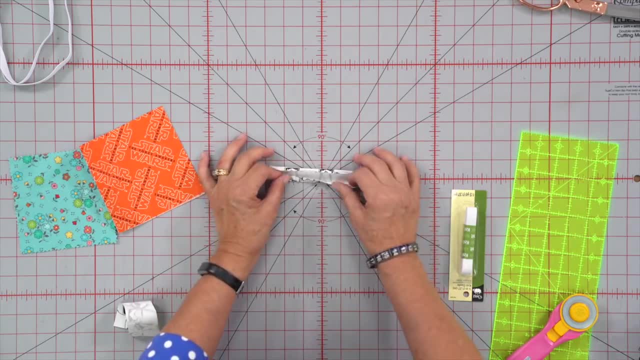 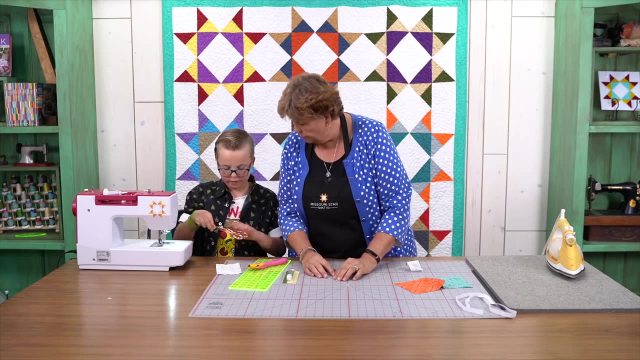 piece right here, And I've ironed the two sides to the middle like this: Do the next, Thank You, And then folded it in half like this: Now what I want you to do, and you have to be super careful about this, oh, do you need? 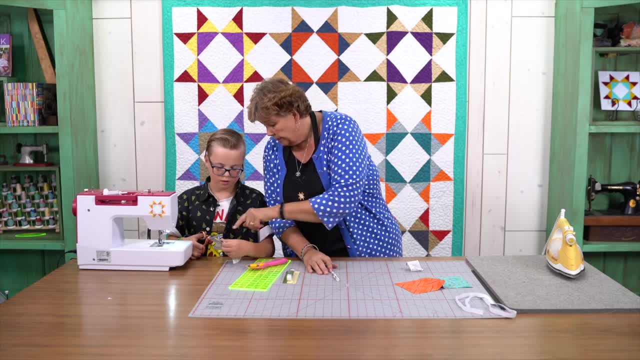 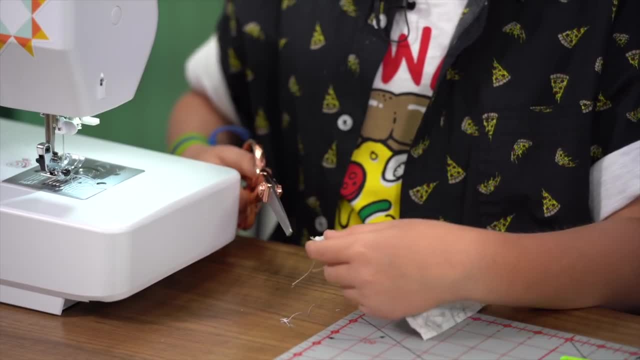 to do some trimming, Yeah, So when you're trimming you want to, just if you just clip that little corner a little bit like just like, yeah, just like right up by that edge, Now can you come and do that in here so we can be sure everybody can see that. 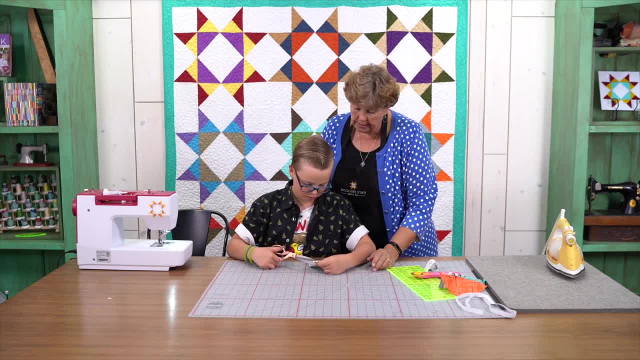 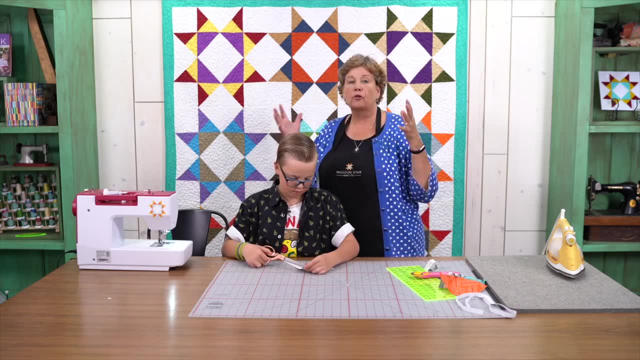 Yeah, Because I have a feeling there's going to be some dapper dressed boys out there just from watching you do this video. Yep, you clip that corner. That's going to make it easier to turn and it's going to make your corners really. 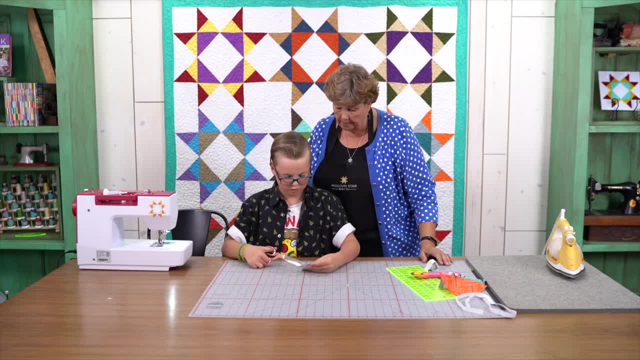 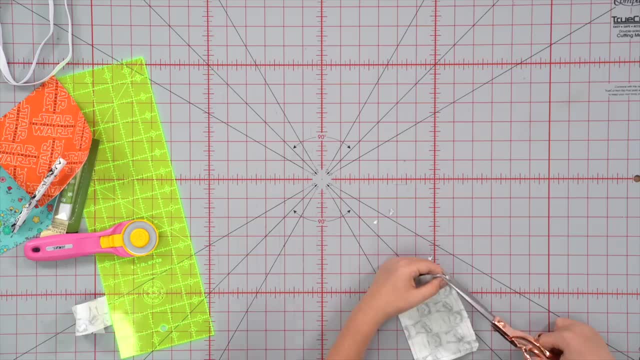 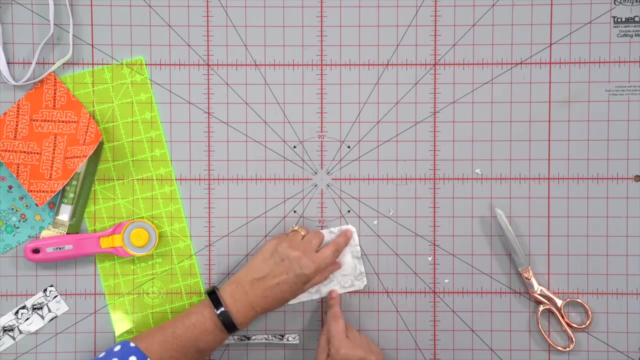 sharp. Ok, Yep, those are the tricks of the trade mister. I didn't know that. That's why you have a grandma. Yep, That's right. Alright, now, right here, I see that you stopped sewing before you hit that edge, and 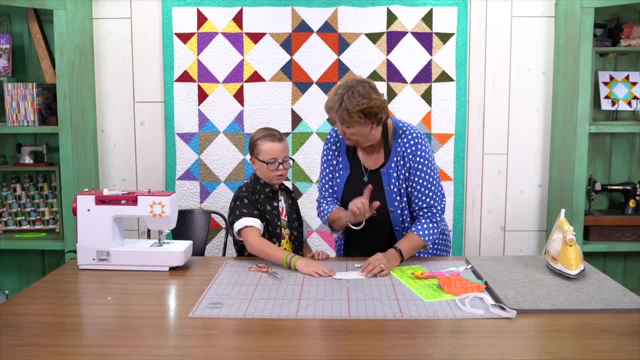 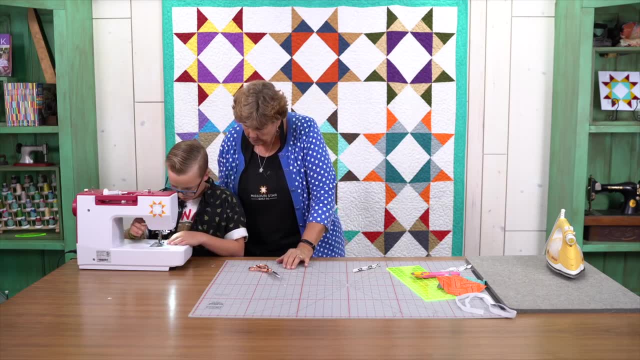 you stopped right here, So you're going to want to go and finish that all the way up on both of those sides. Alright, So, yep, like I. just what I would do is I would turn it this way and I would line that up like that. 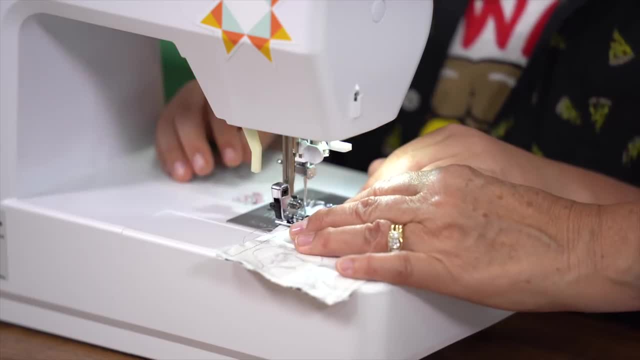 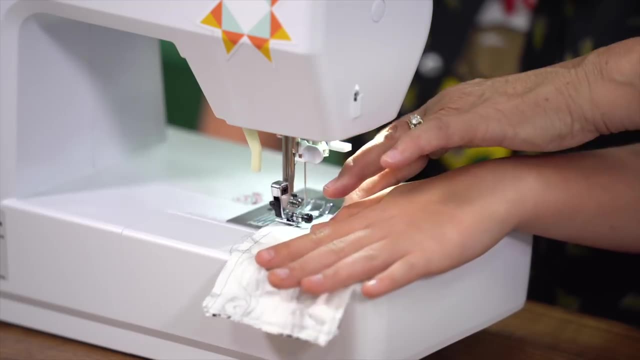 and set your needle down in the stitch like this: so let's look where it's actually going to sew, Alright, And then just go ahead and sew off all the way off that end. There you go, And then over here another one too. 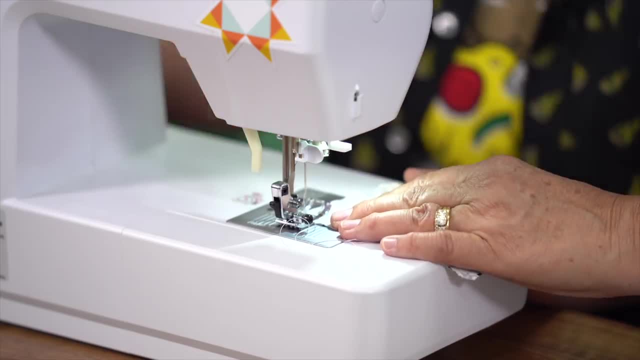 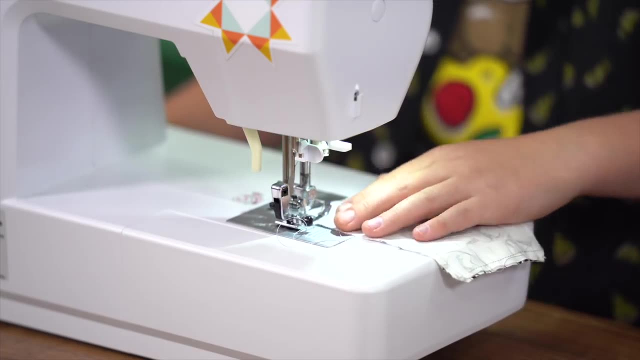 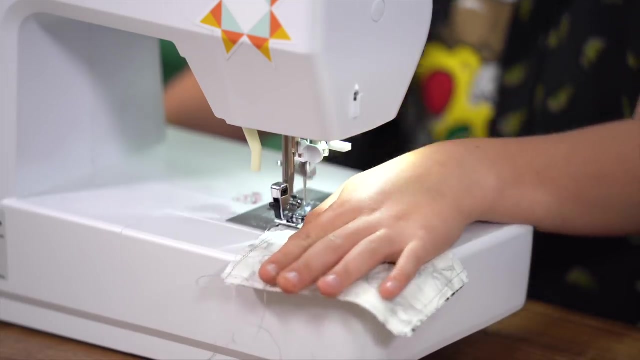 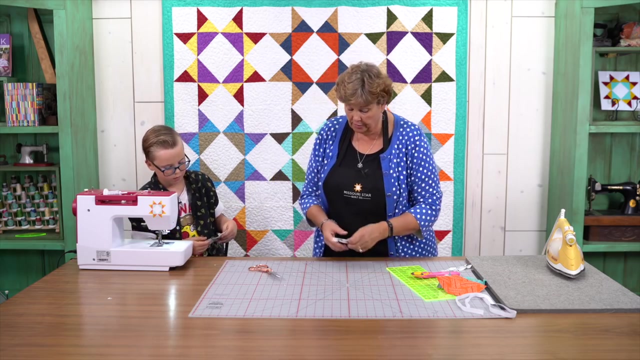 So like this: Alright, And then just sew across there, Yep, All the way to the end. And then There you go, Perfect, Alright, These little sewing machines have a nice little cutter on the side. Alright, now what you're going to do, this is going to make the little band that we're 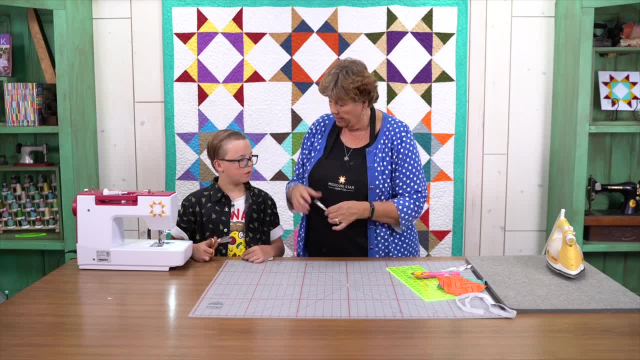 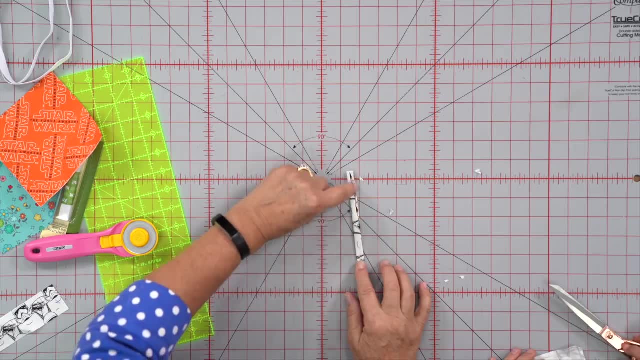 going to put around the center of the bow tie to make it swinch up in the middle, Yep. So what I want you to do is I want you to sew a stitch right along this edge, right here, Just pretty close to the edge. 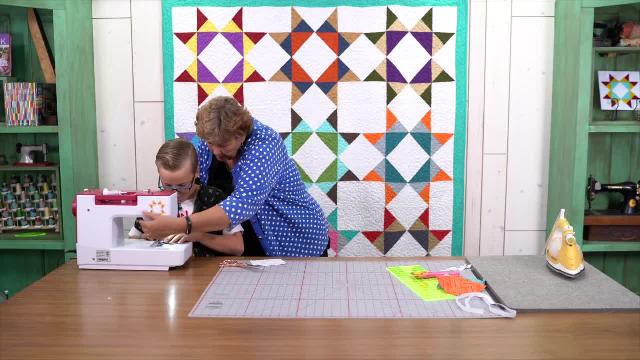 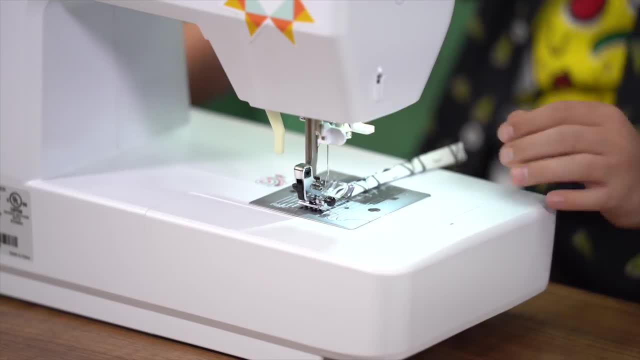 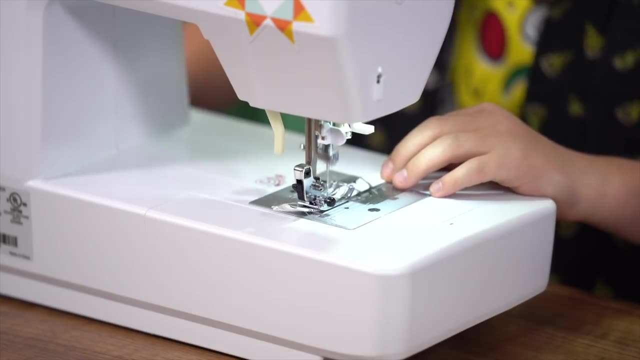 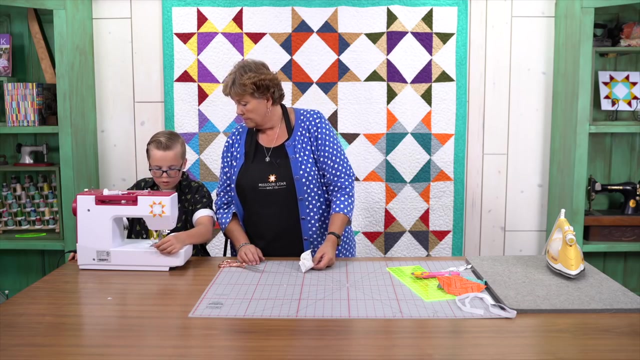 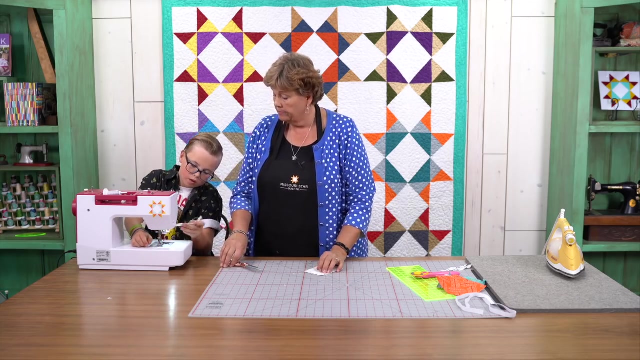 Okay, Alright, Sew right here. Yeah, I would, yeah, just go ahead and sew right there Like one one, like one, sew right down the middle. That's good, Perfect, There you go. Alright, now you can clip that off. 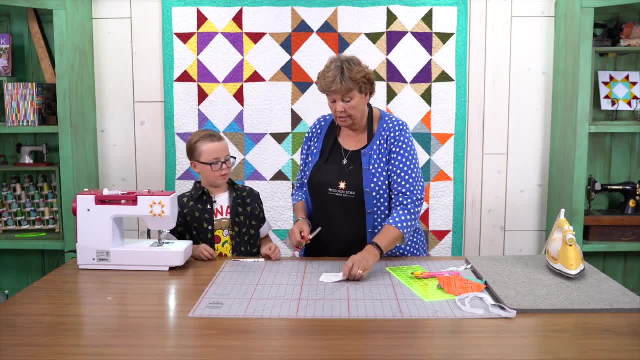 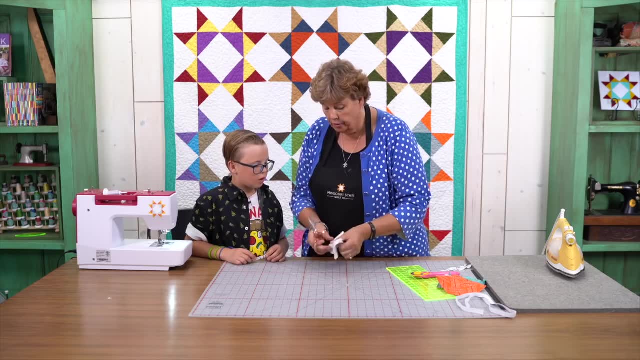 Alright, the next thing you need to do is you need to take this bow tie right here, Yeah, And we need to clip this. and see, I pulled the fabric apart, so I'm only cutting one side and make a little cut like this, Yeah. 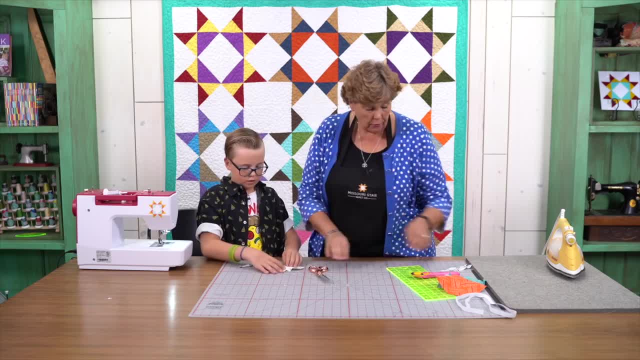 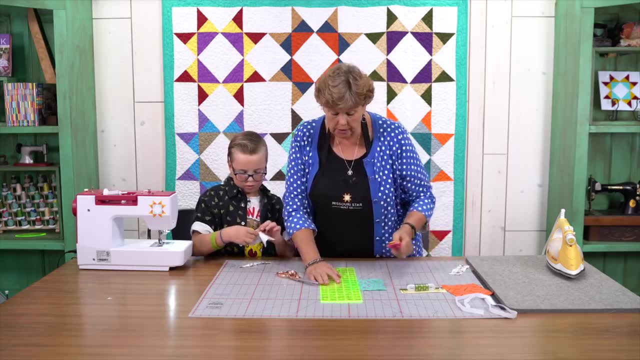 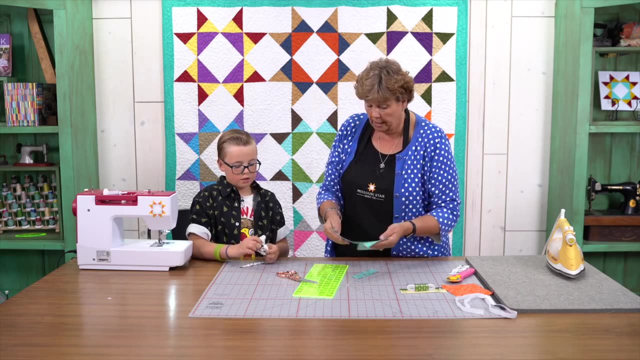 So you can now flip it inside out. So I want you to turn that right side out. Yeah, I remember doing that. Yeah, Now, while you're doing that, I'm going to go ahead and I am going to cut a piece off of this flowered one, because I think it would be fun to make Ashlyn a bow as well. 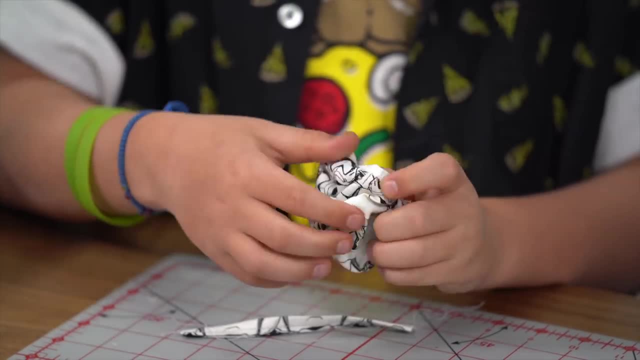 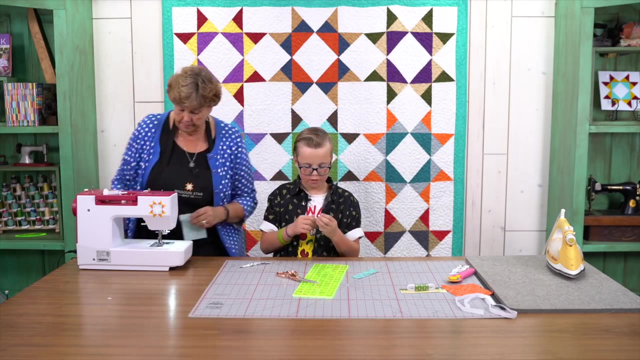 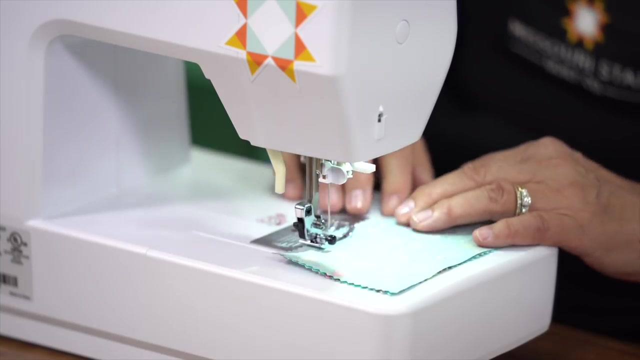 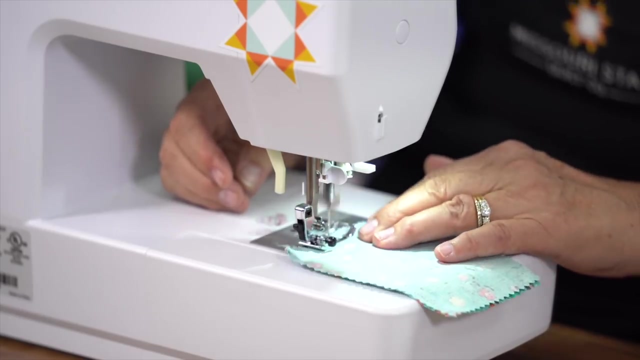 And while Ashlyn won't wear a hair bow, these work perfect. I mean a bow tie, these work perfect for hair bows. So I'm going to sew this around while you're doing that, Ready, And I'm just going to go super fast. 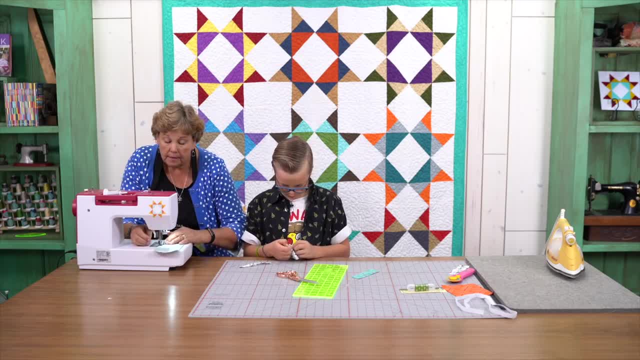 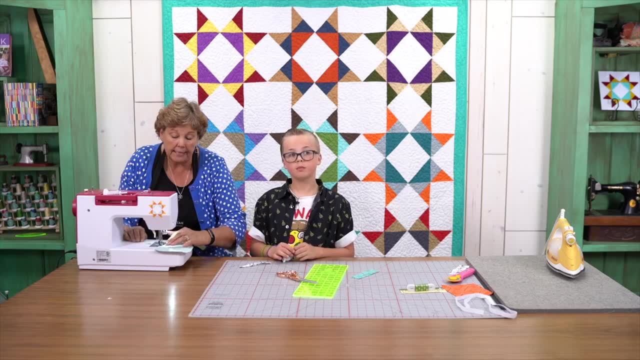 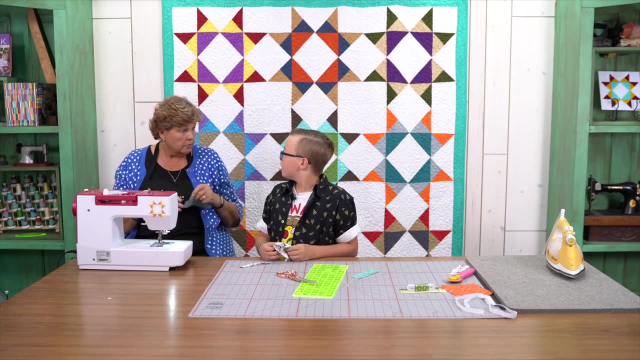 Now, it really doesn't matter what your seam size is when you're making these bow ties, because it just depends on what size you want to end up with, right? Yeah, So you could actually make a giant bow tie if you wanted to. Whoa. 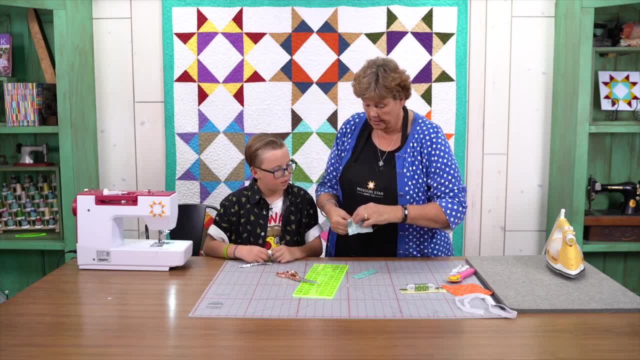 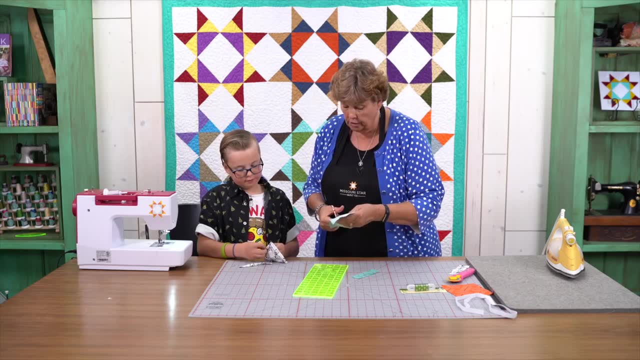 Yeah, Pretty cool, huh? Yeah, Alright, now I'm going to make a little cut right here. Yeah, So I can turn this one too. Now, when you get your thing mostly turned, what I want you to do is I want you to take. 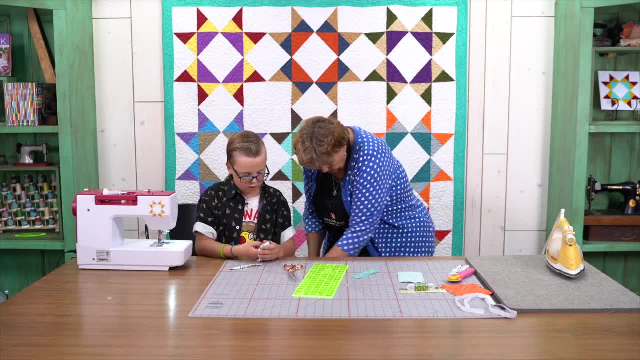 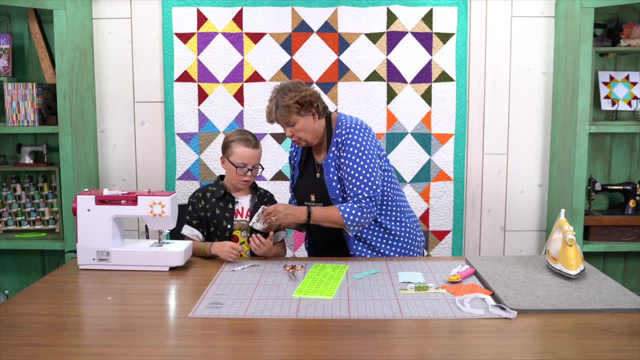 a little turning tool like we have a. we have a little. we have all kinds of little turning tools. We have all kinds of little things you can turn with. I like to use like a little pencil end and just push it up in the corner and push the. 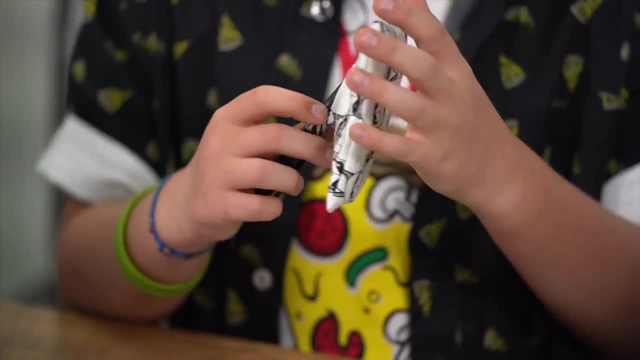 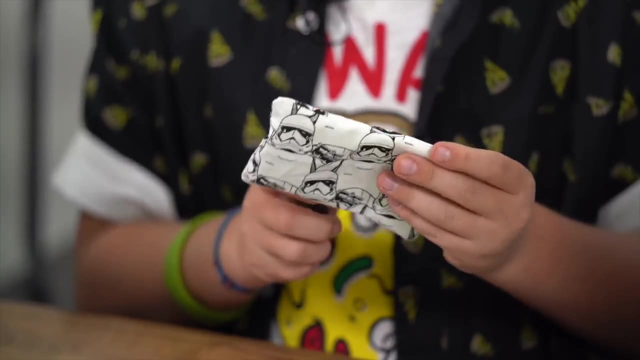 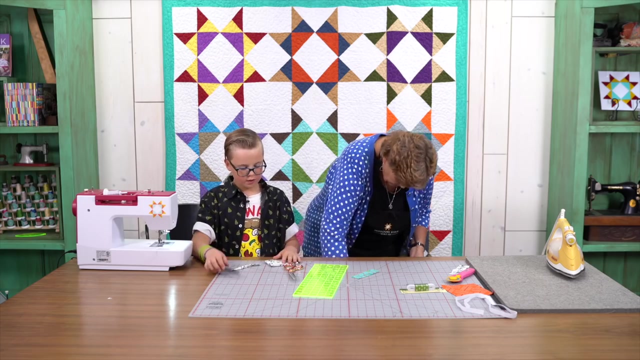 corner out like that. Oh wow, So do that on all four corners, And I'll turn mine too. We'll just make this work. That helps a lot, Doesn't that help a lot? Yeah, And I have a little. oh, I'll use yours. 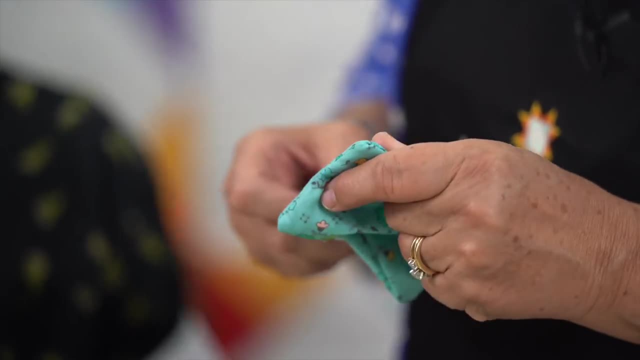 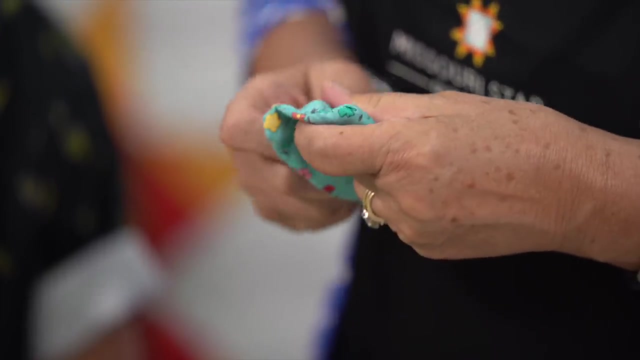 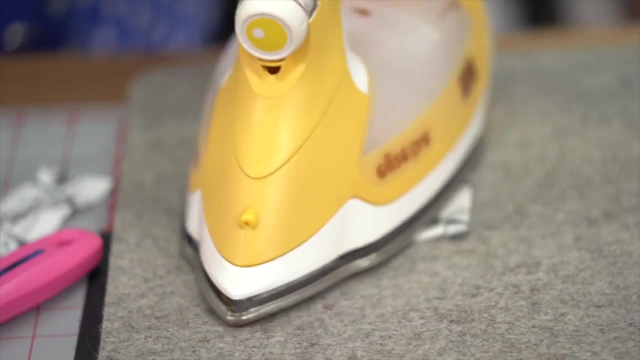 Ok, Alright, So now. So we need to put the middle part on there, Ok, Let me see, hang on just a sec, Alright, So So let's press this. Let's go ahead and press this, Ok, And you'll notice there's still a big hole on the back right. 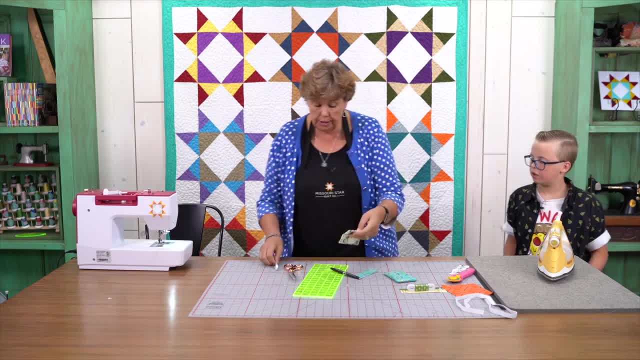 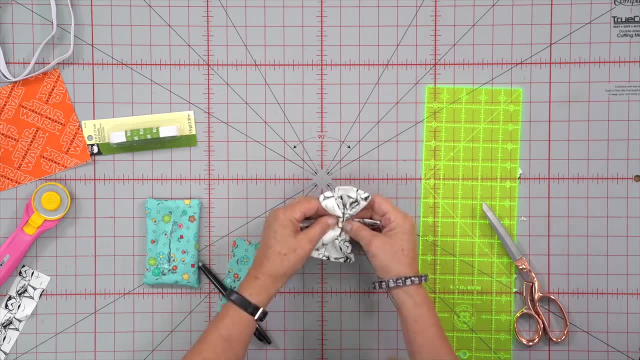 Yeah, But we're not going to worry about that, and here's why We're going to put this middle band around it right here, just like this, And this is going to all get squinched up like this, Yeah, And then we're going to just pull this band. 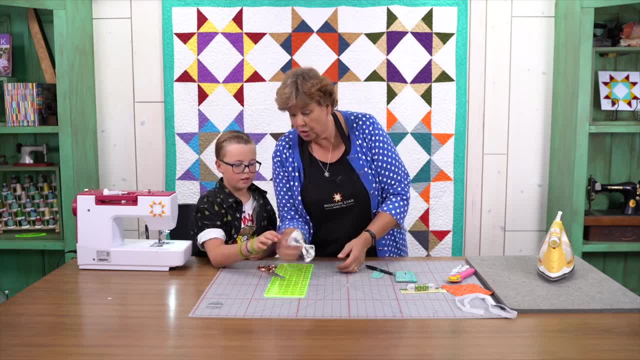 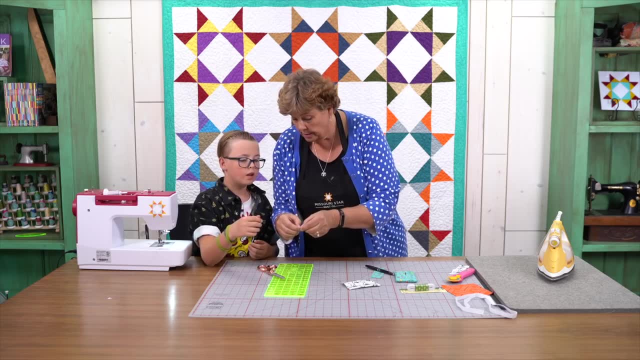 We're going to see how tight we want it like about this tight, Yeah, Does that look like a good bow tie? Can you see how fast that went together? Alright, I'm going to slide this out And I'm going to have you sew right across here. 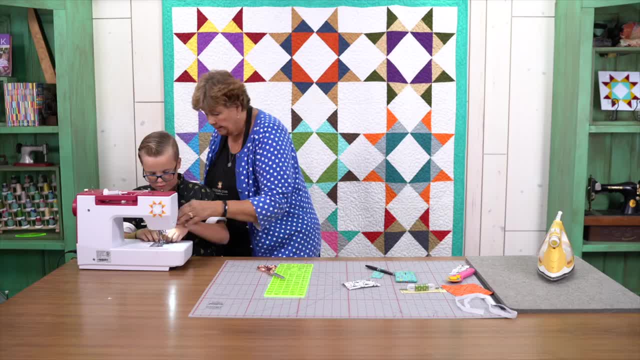 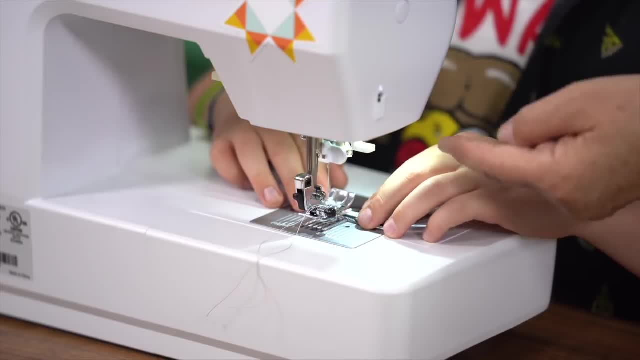 Ok, So right there, Yeah, Let's. it's probably easiest if you a little bit more room, A little bit more. No, the other way, That way, That way. There you go, And then you're going to sew. 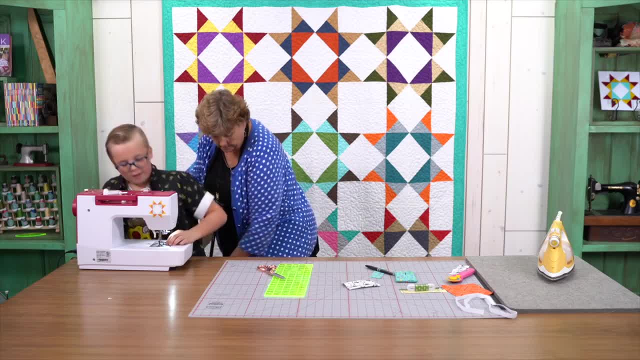 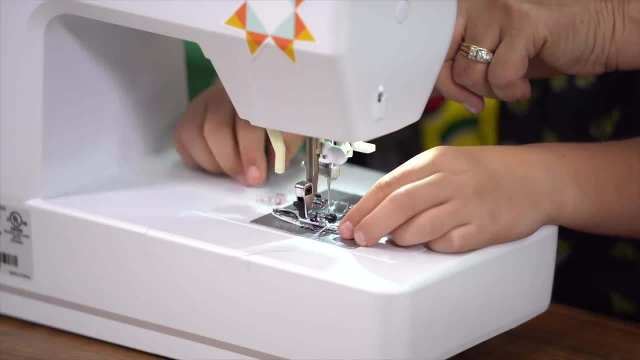 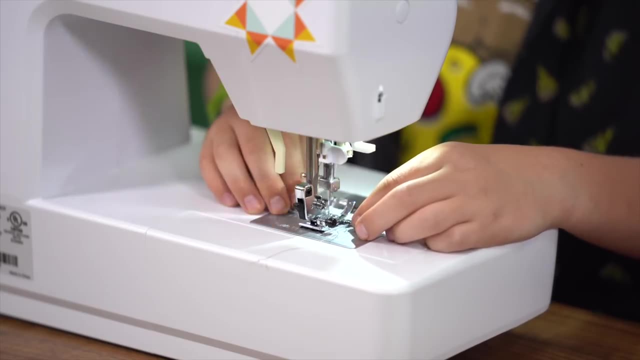 And we probably need to move this forward now, don't we? Yeah, I got longer legs than you, but not forever. Alright, now stop, And then you're going to push this backup button and sew back and they're going to go forward. 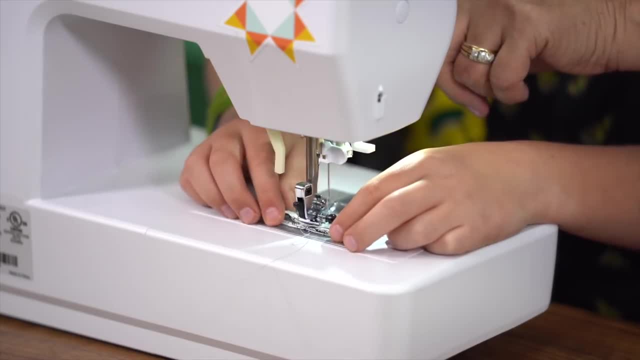 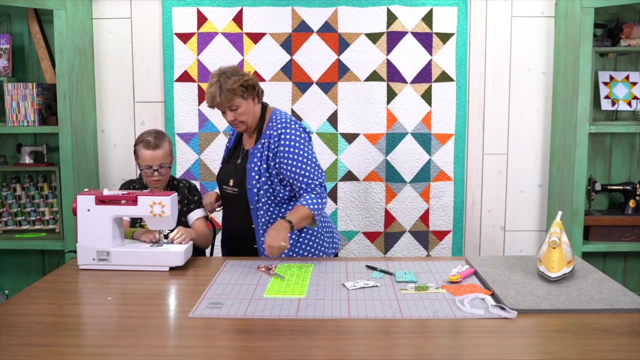 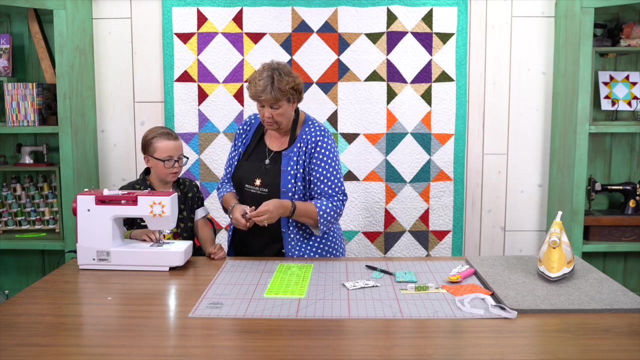 And then we'll stop and we'll go back. We just want to make sure it's really secure. Alright, now let's open it up up. We'll trim this all up, because we don't want any of those threads or fluff, And then what we're going to do is we're going. 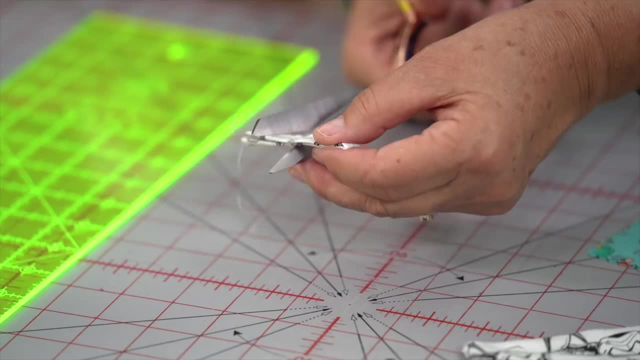 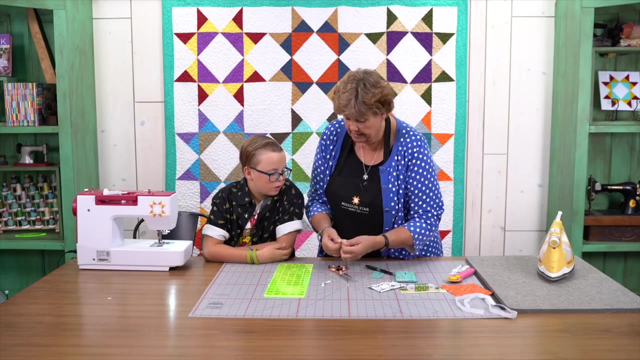 to trim this about a quarter of an inch from where we sewed it. Ok, just like that. Alright, now we're going to flip this right side out like this, And it just makes this little ring. Ok, Then I want you to push this through, And what we're going to do is we're going 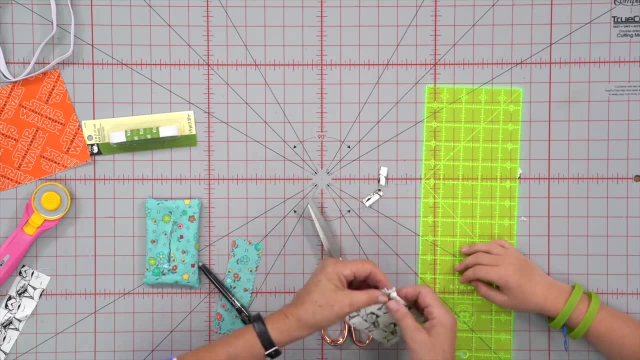 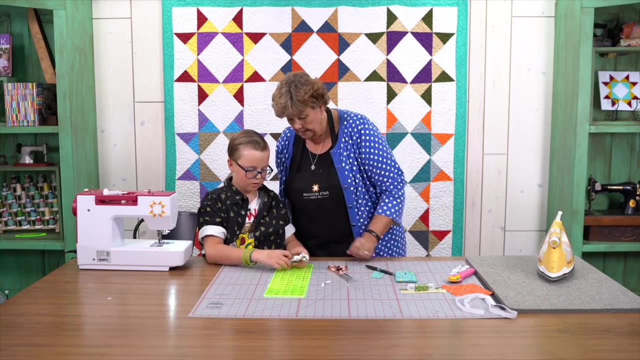 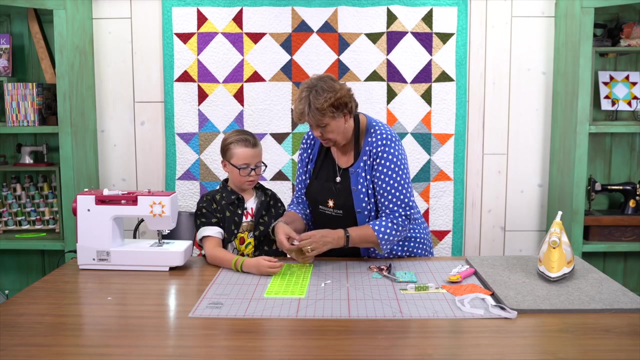 to start with the seam part in the back by this seam part, And we're just going to pull this in like this. So go ahead and pull that through There. you go Now center it up in the middle like this: Ok, Make sure these parts flip up right here, So we kind. 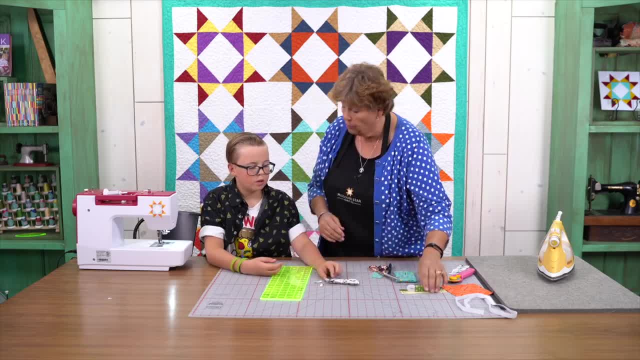 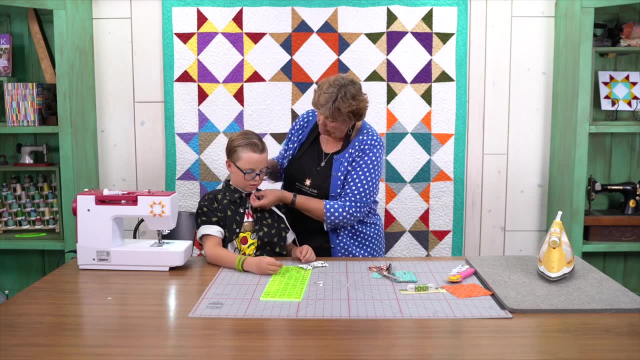 of have to do it two handed and we flip up. Now all we need to do is add some elastic so that this will fit around your neck like this. So we're going to kind of loosely measure your neck, because shirts aren't exactly the size of your neck. They're a little bit bigger. And then what we're going to? 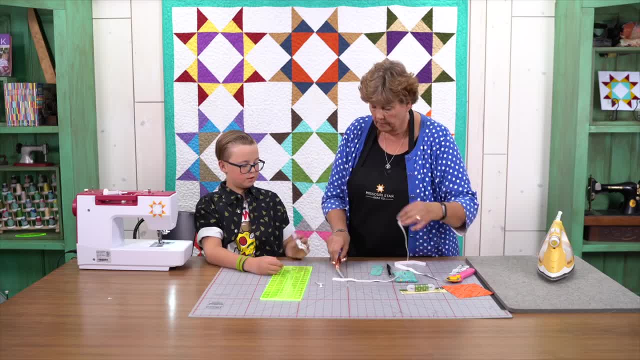 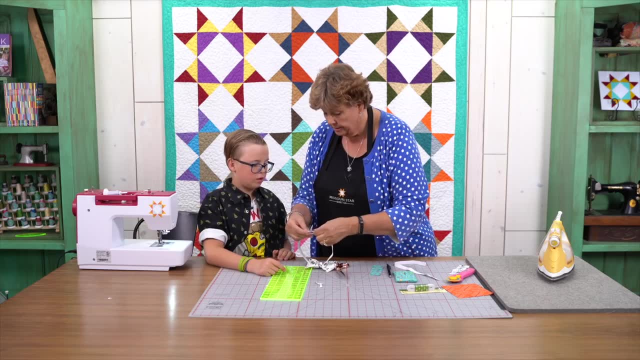 do is: we're going to put this through, I'm going to cut it, We're going to slide this through here like this: Ok, Just like that. And then we're going to sew this end together And we're going to sew it flat, So we're going to overlap it like this, Just overlap. 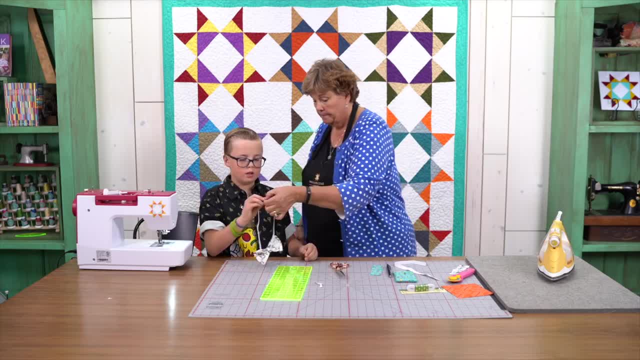 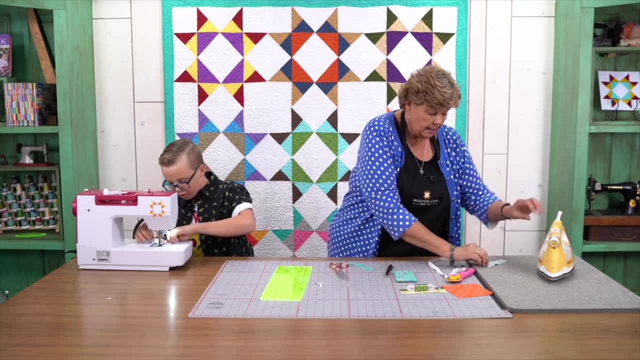 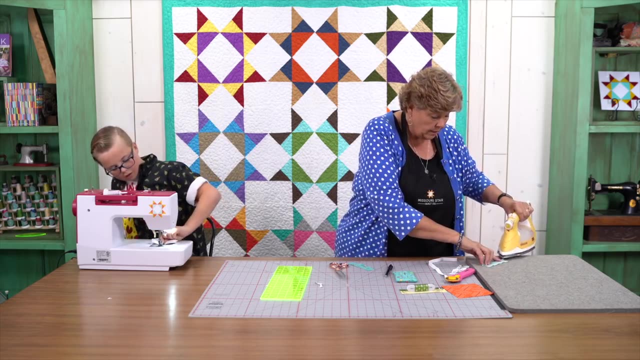 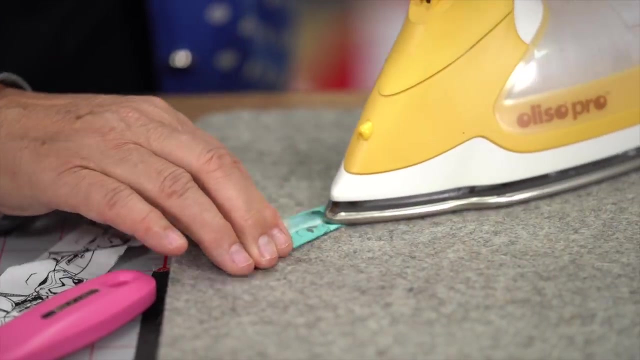 it And we're going to sew one seam right down the middle. Ok, Ok, And that is completely adjustable. So if you need to change that so that it's tighter, super easy to do. Alright, I'm going to iron this middle over here, You good. 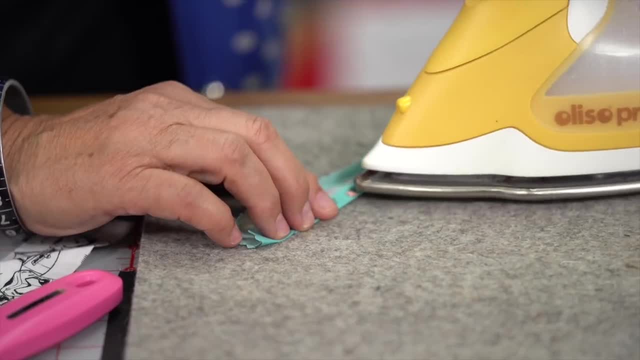 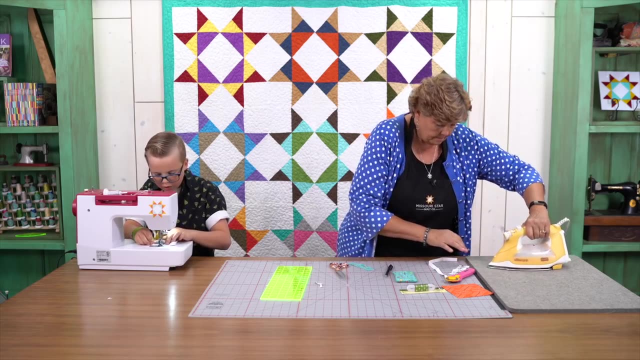 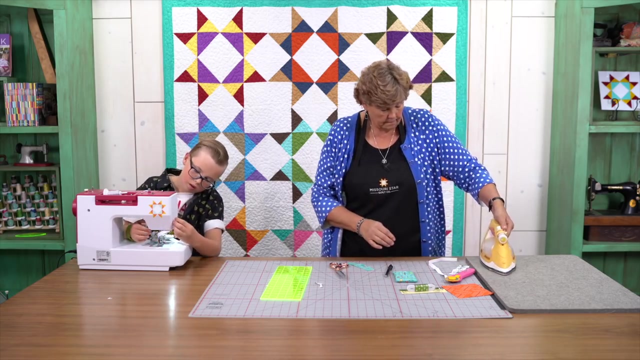 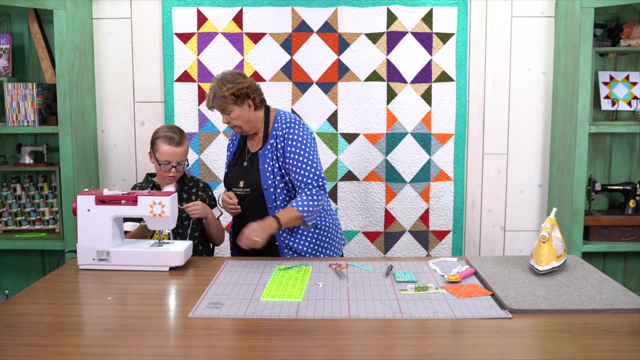 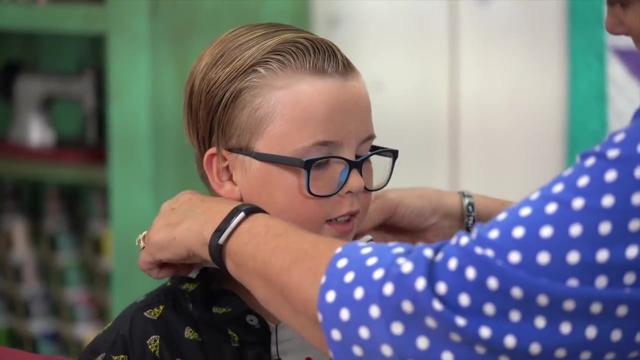 Yep, I heard a little clunk. As long as you're ok, Ok, Underneath Did it stick, Perfect, Alright. so now let's look how this looks on you. We're going to put it over your very carefully done hair. We're going to tuck your little collar under. 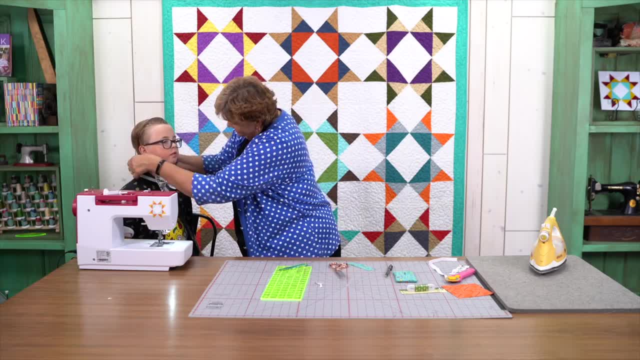 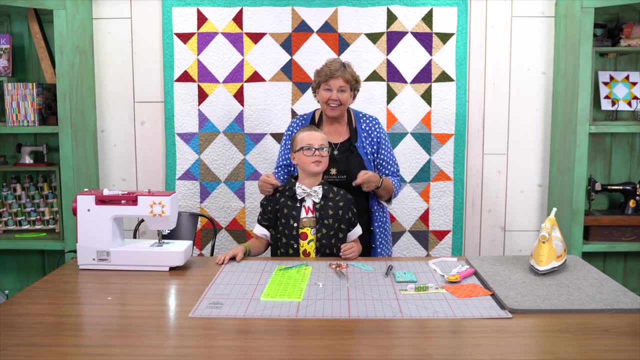 here, And I would actually probably make this bow tie a little bit smaller, But it looks. it looks so cute. Come out here where everybody can see you. Can you see this? How cute is that? Alright, let's quick finish up one for Ashlyn so they can see what it looks like. 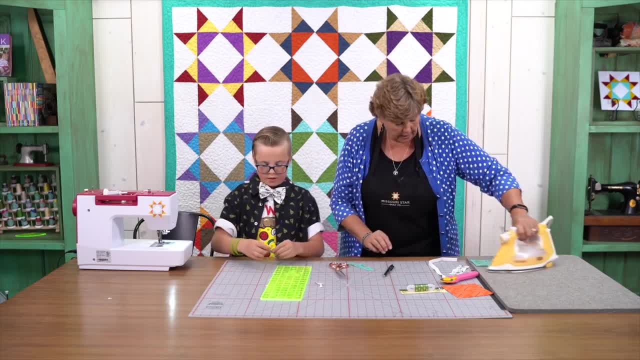 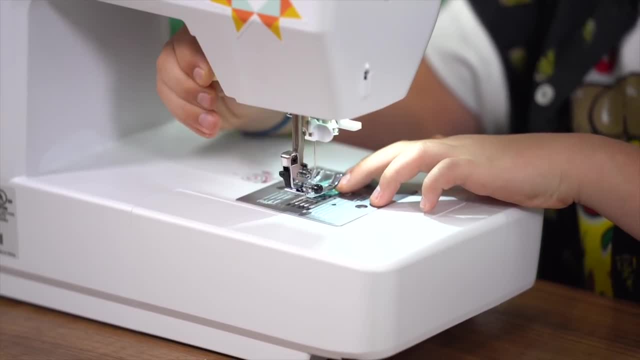 as a hair bow. Ok, So this right here, we need to sew a strip down the middle. Ok, We can't tell her, it's going to be a surprise. alright, Okie dokie. Now if Ashlyn needed a big hair bow, you know Ashlyn, good sister, Ashlyn is. 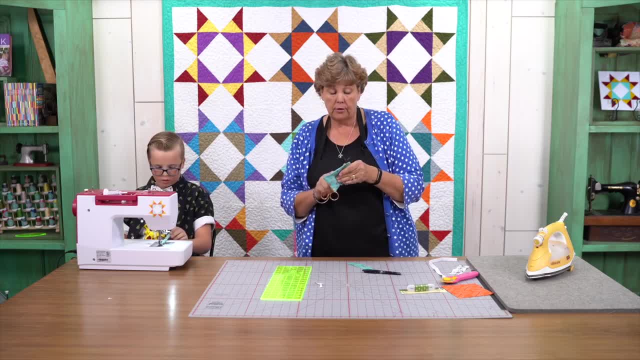 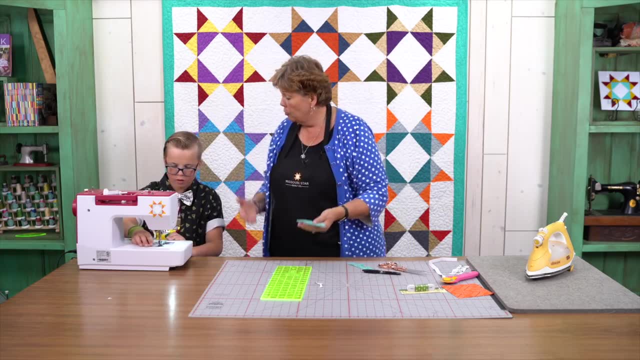 a cheerleader And sometimes they wear big hair bows in their hair And she can make big ones out of this. Just change the size of your square. If you use a bigger square, you're going to get a bigger bow or a bigger bow tie. 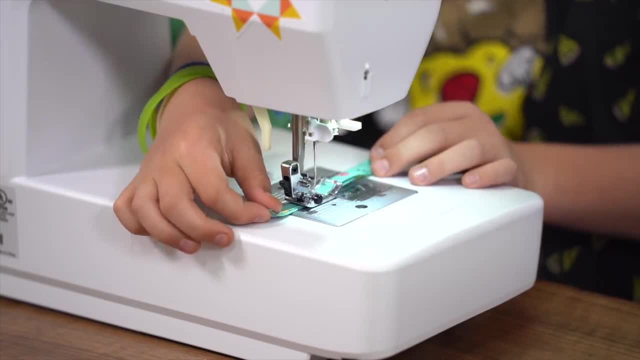 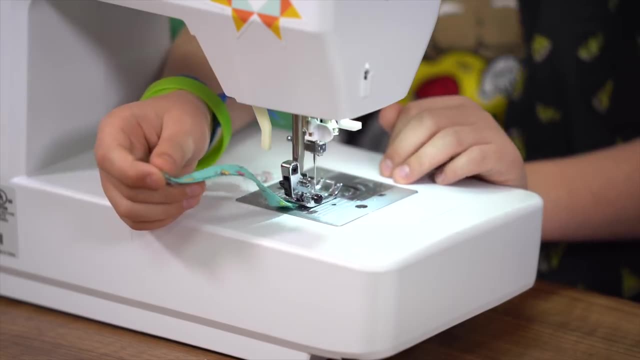 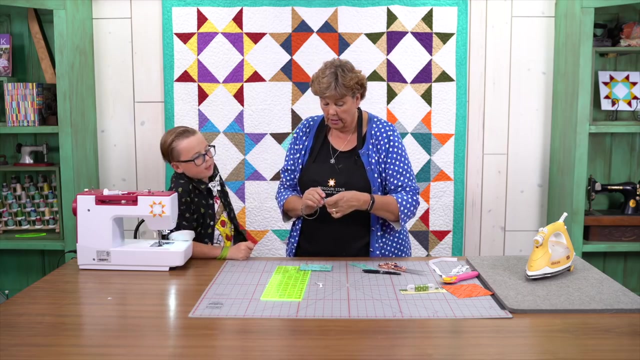 Oh, it came off. You know what? it's ok if it came off, because here's why We're only going to use a little piece of it to squinch it up. Oh yeah, Remember. So let's go ahead and we'll. 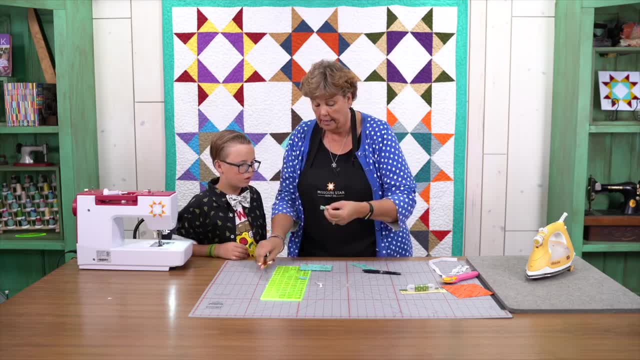 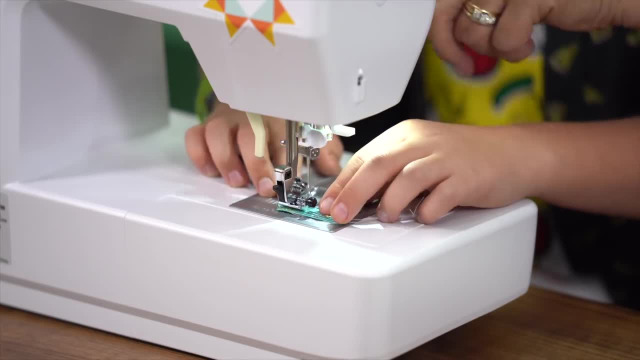 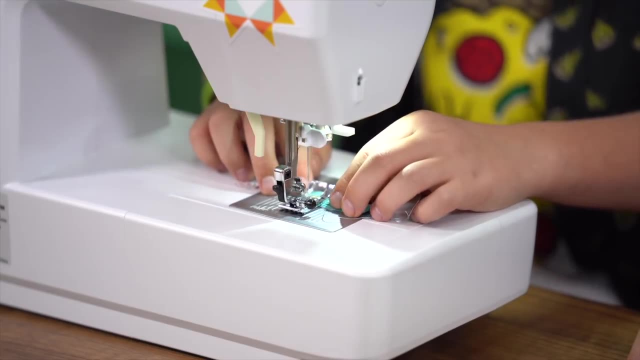 sew this right here. As a matter of fact, I'll cut it first and let you sew along that end. Ok, So just sew on the side where the fold isn't. Now let's go back. This is the back up button. Now go forward. There we go, That's. 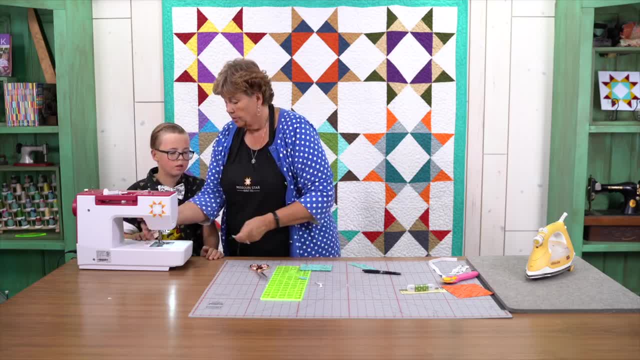 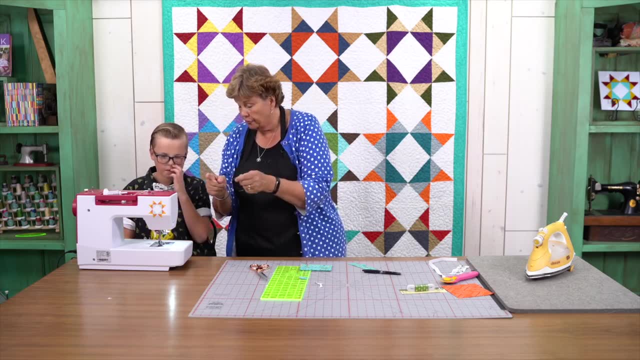 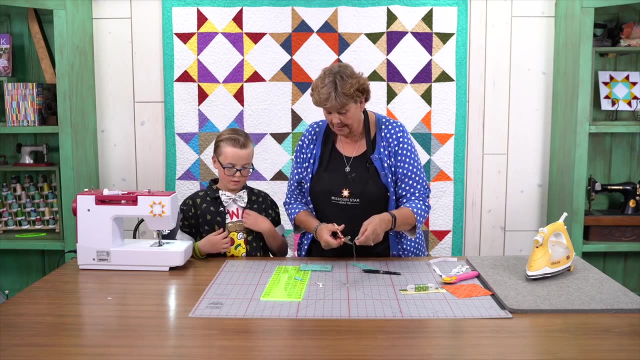 probably good. So it's always easier to have the thread pull through if you lift up this presser foot, because that the presser foot is attached to the tension rings that they. that's what makes it tight. Yep, You knew that? Um, I didn't. 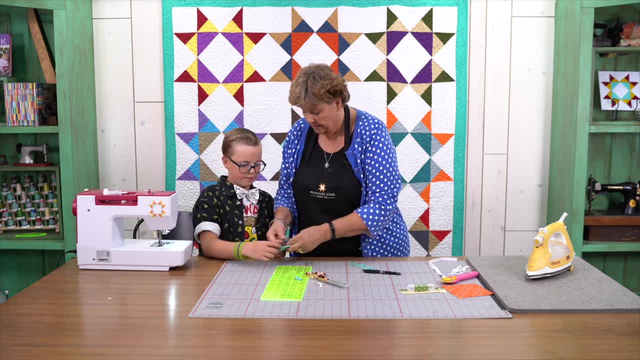 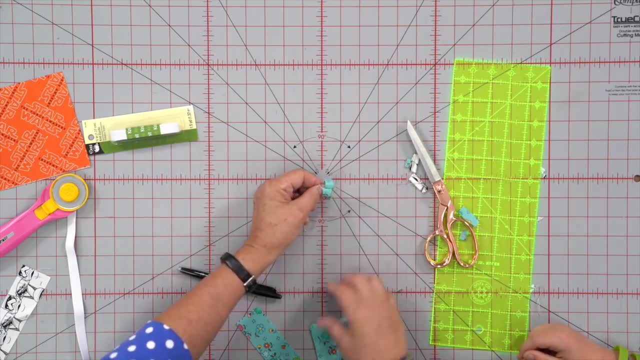 Alright, so let's pull this through here. Remember the: the fold is in the back. Now even this: take a look at this. See how this is just a little bit off. Yeah, It's not going to matter because it's on the back. Yeah, 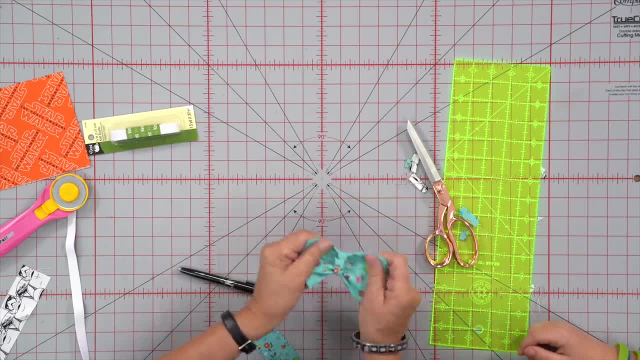 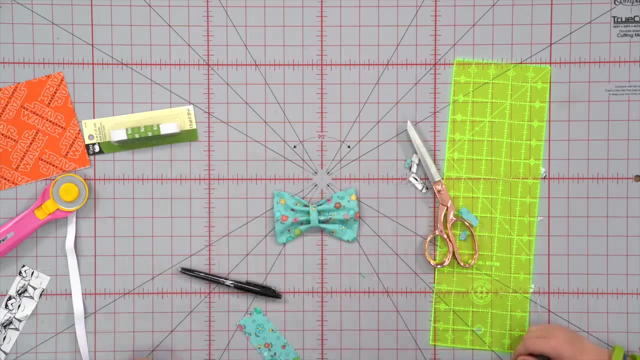 So we're going to push this through like this, Ok, And then we have this cute little hair bow. We could make that a little bit smaller, Yeah, A little bit tighter, if we wanted to. As a matter of fact, let's do it, Let's do. 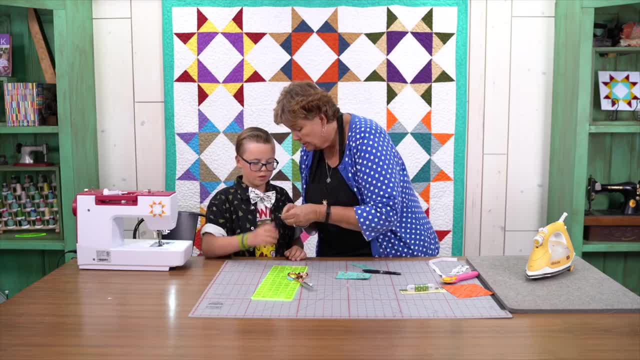 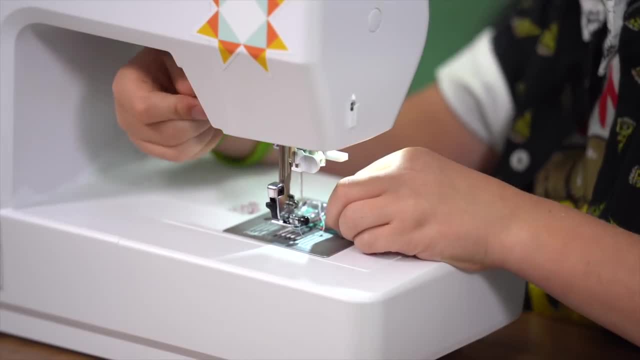 it real quick. Just take this seam in just a tiny bit further. ok, Can you do that? Yeah, And I'm going to get a piece of elastic, And this is how your elastic comes. You usually buy it in a package like this And you can. 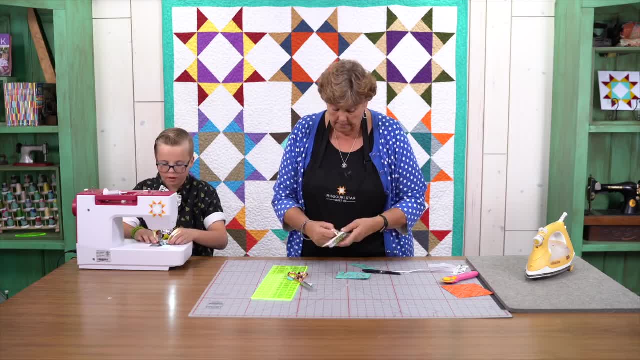 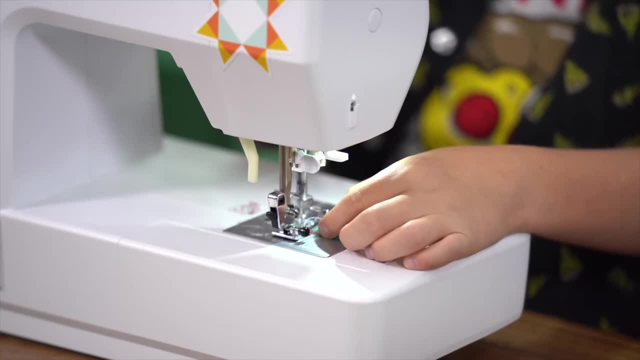 just take it off and it comes. There's a- I don't know how much is in here- One and a half yards, you know. So that's quite a bit. But because now, if she wanted to make a ponytail, 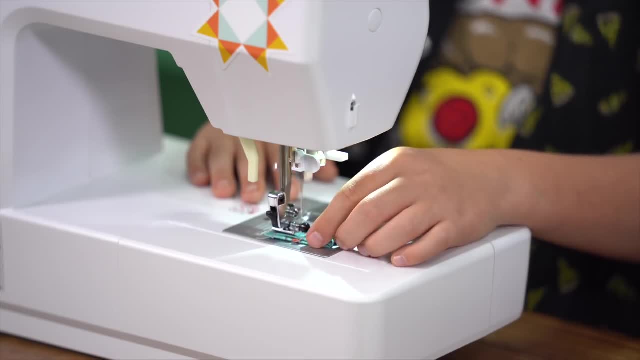 If she wanted to make a ponytail out of this, that would be a little one. If she wanted to make like for her whole head, that would be a big one too. Do you think she wants a whole head, bow or a ponytail? 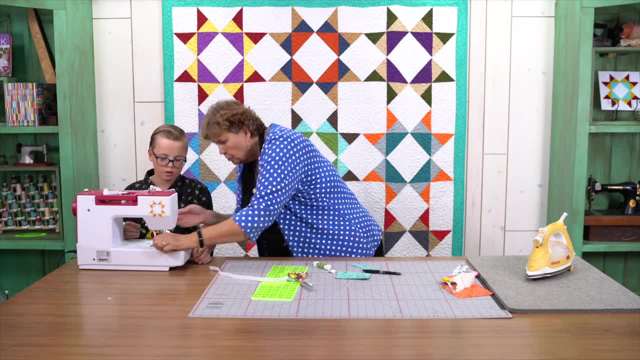 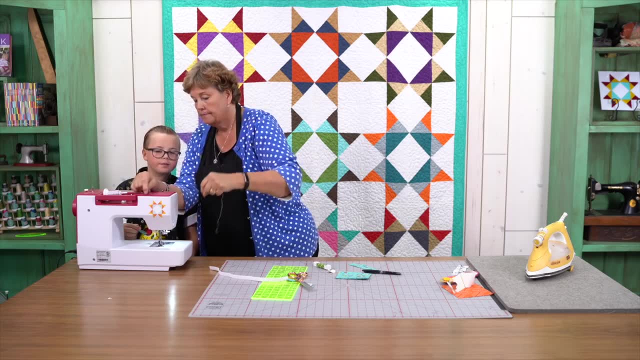 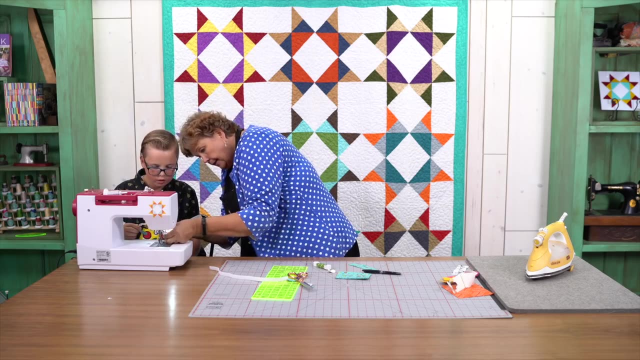 Oh Oh, you know what happened. Your thread's unthreaded. Uh oh, That's alright, That's an ok thing to happen. It just happens sometimes. So you just follow the directions on your sewing machine. Most of them have little arrows. 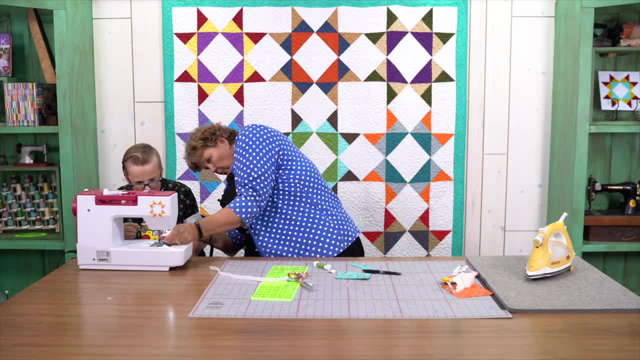 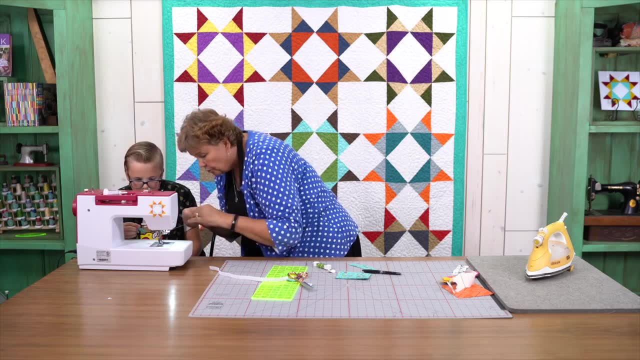 And then go right down here. Ok, Go through. And then you have to have good eyes to be able to thread that needle. And, uh, your grandma's, your grandma's eyes aren't so great anymore, But let's see if I can do it. 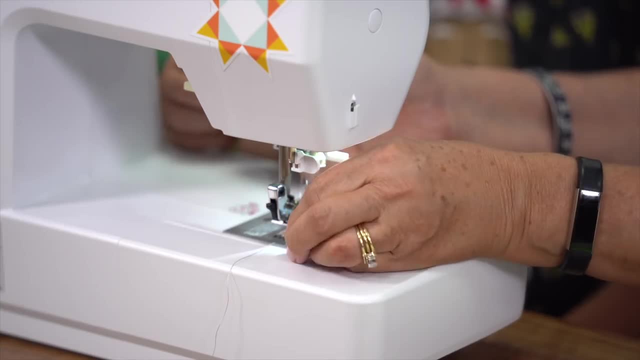 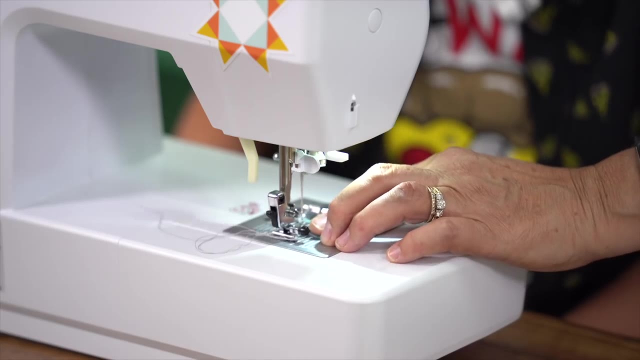 First time. Oh yeah, Oh yeah. Alright, Let's sew this one more time. Let's just go in just a little bit like this: There we go, There we go. Now we're going to go backward And go ahead and push. 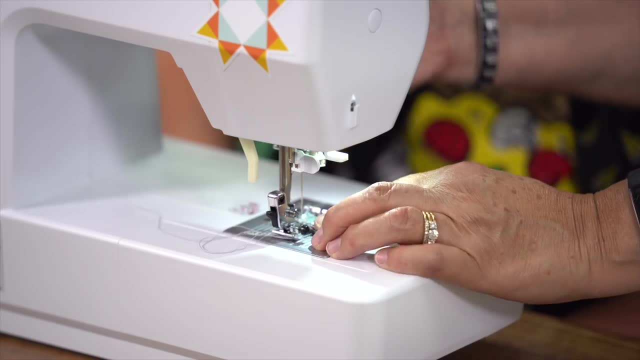 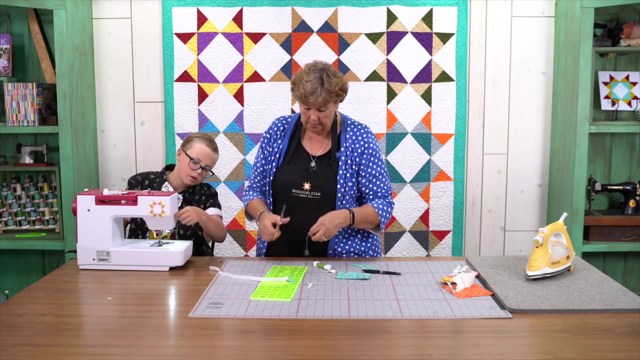 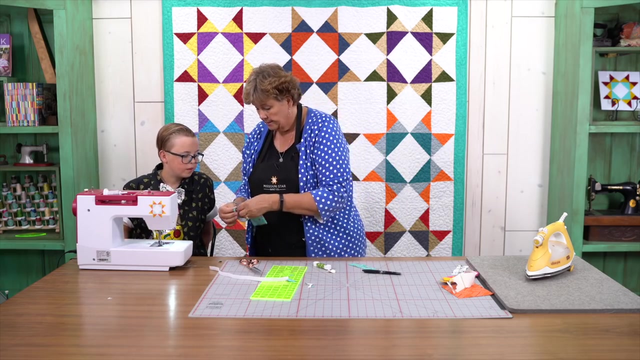 the foot. Alright, Perfect, Alright. now all these places that we sewed. this is never coming apart because we got so many little seams, But we're going to take this now and I'm going to have you slide this through here like this: 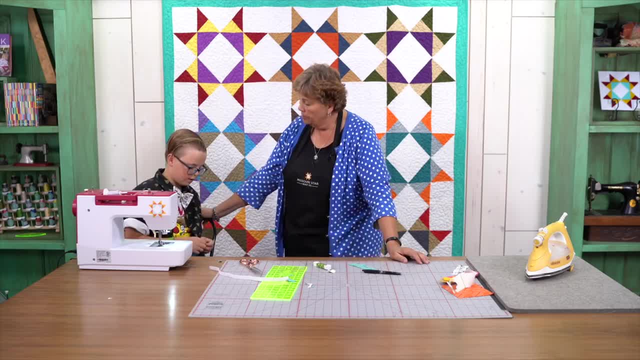 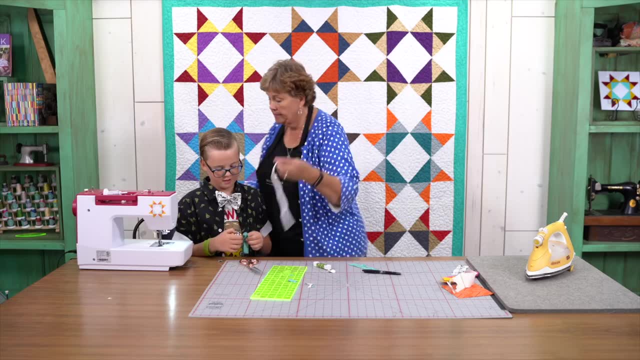 Alright. Ok, Now do you think she'd rather have a ponytail, hair, bow or a whole head? one, A ponytail, A ponytail. Alright, I'm going to sew this together to make a little ponytail, But I can't actually sew it until we have the bow tie ready. 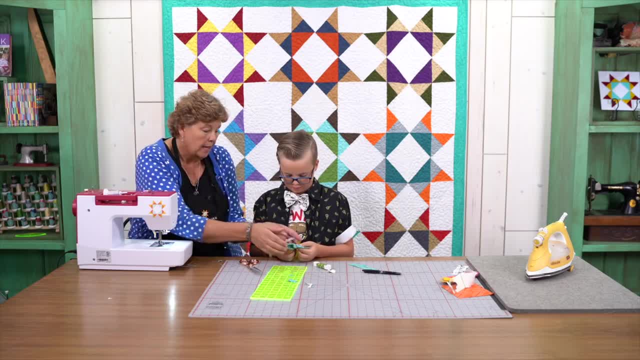 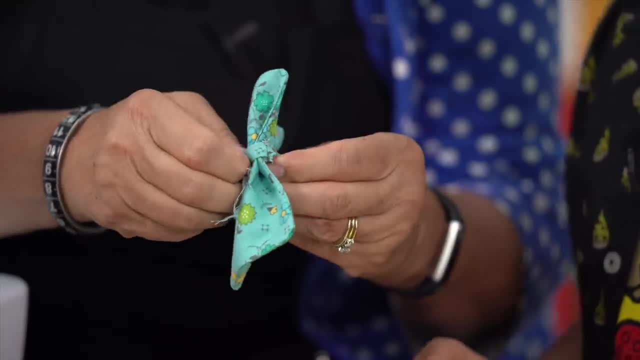 Yep, We can't call it a bow tie. What do we call it now? A hair bow. Alright, Now I'm turning this over, so the seam is on the inside And centering it up on the back, where it has the open place where we turned it, because you'll never 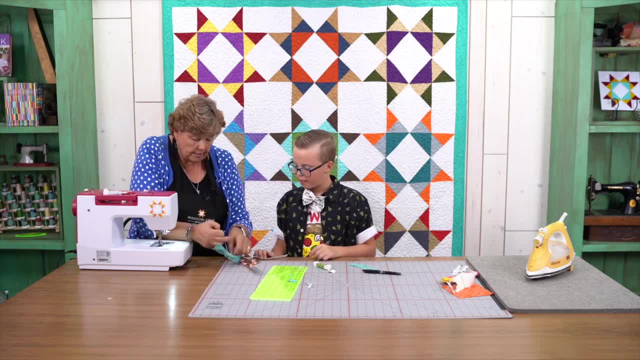 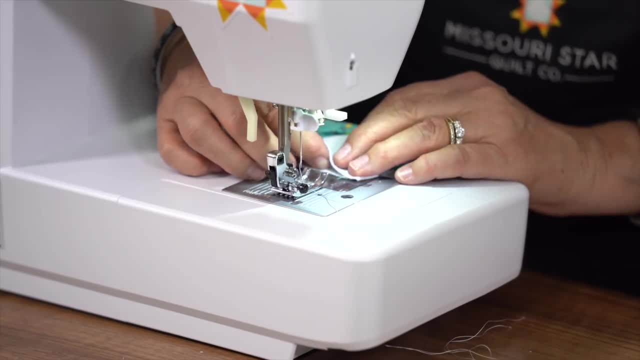 see that back, And then we're sliding it in here like this And I'm just going to make her a little ponytail like this. Alrighty, There we go. Do you think she's going to be excited about this? Yeah,